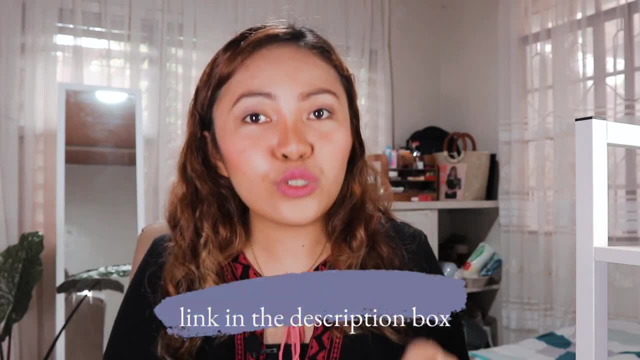 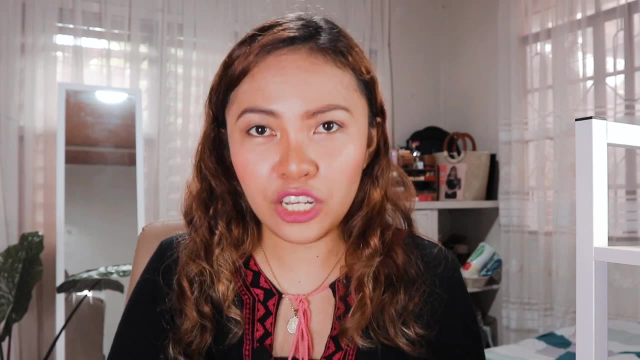 printed out and cut the number cards one to 25.. Once the time is up for them to write the answer, this is now the time for you to draw those one to 25 number cards, And when a number is drawn, the student will use one of the bingo markers, which should be a cereal, jelly, beans, pom-poms. 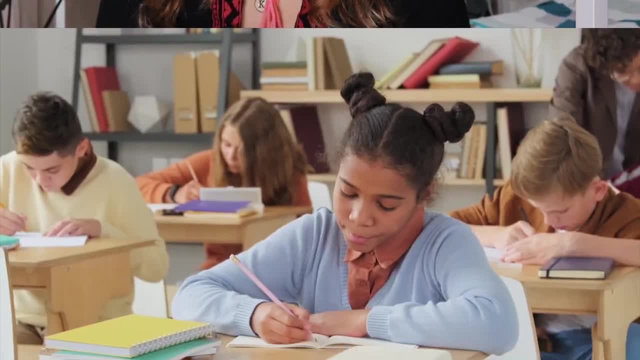 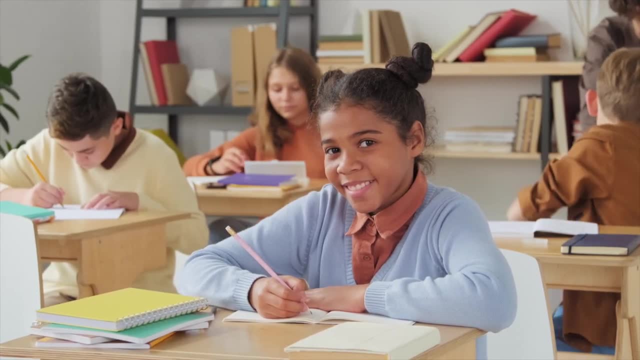 etc. in order to mark the bingo card. It's really up to you what pattern would make up a bingo, but just make sure to state that one at the beginning of the game. Just an extra tip: if you have lower level kids, you can use. 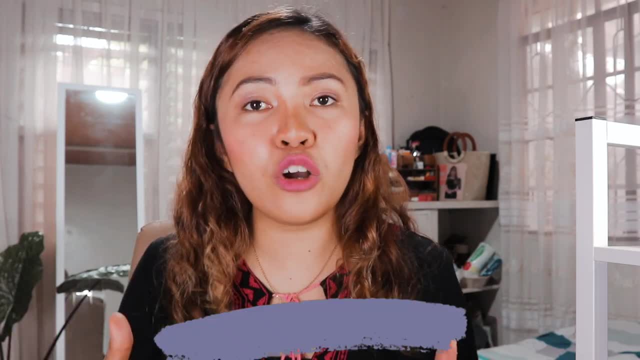 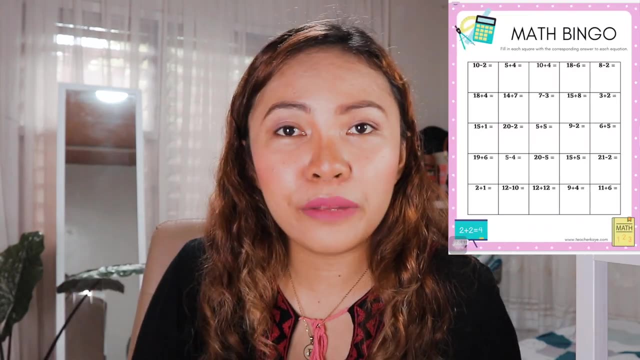 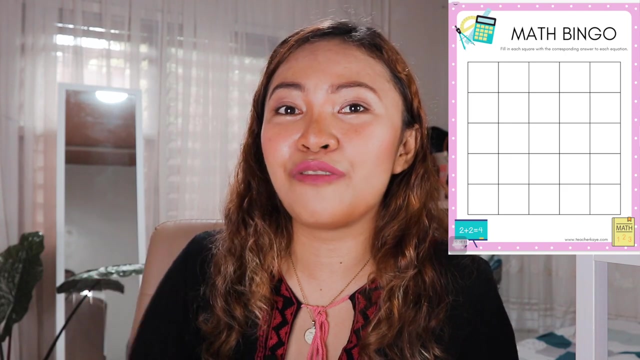 addition or subtraction for the equations on the bingo card. But if you have higher level kids then you can also use multiplication. The ones on my template are addition, subtraction and an empty one for you to edit Again. link is found in the description box. 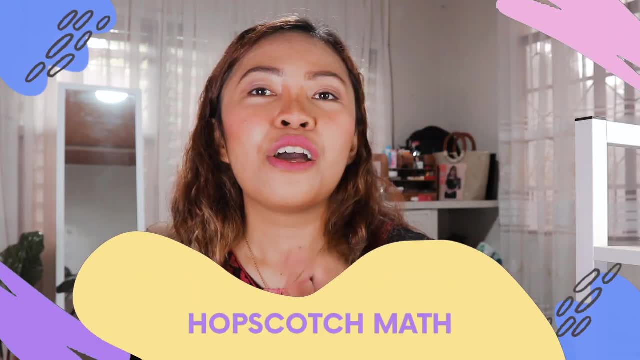 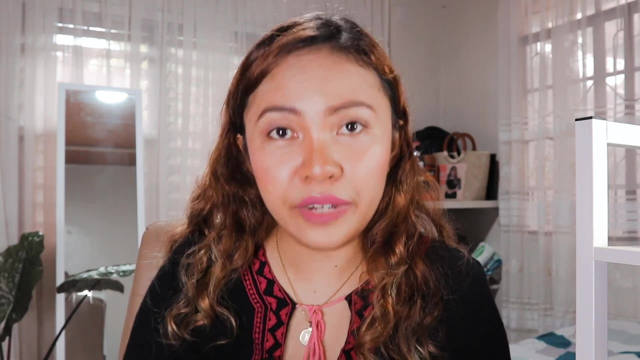 down below. The second game is hopscotch math. This game is a great way to get your students outside on a nice sunny day. Draw a hopscotch grid on the pavement mimicking a calculator layout. Ask the students to form a line, and one by one. 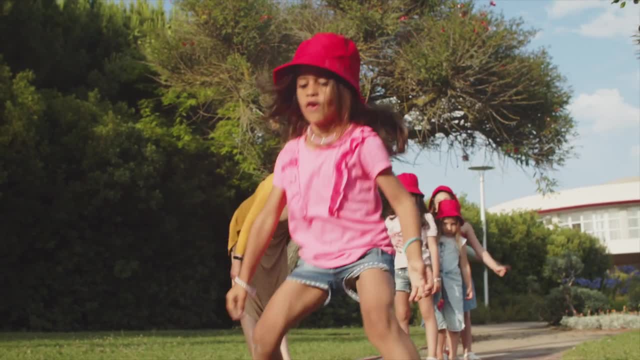 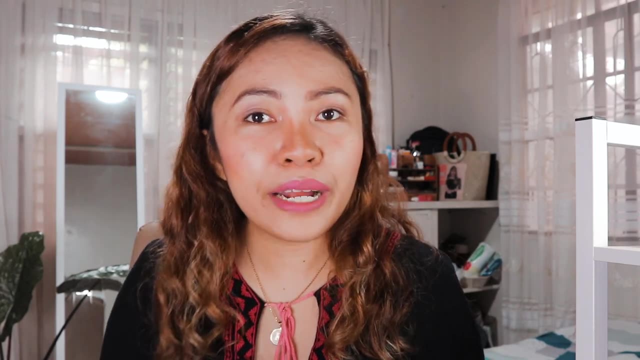 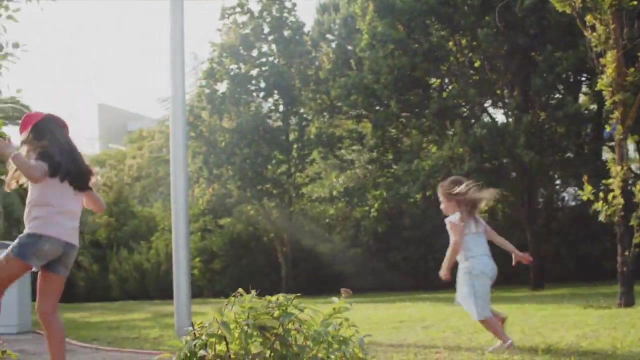 give them a simple operation such as 2 plus 3 or 5 minus 0., Hopping on each element of the equation in the correct order, landing finally on the correct answer. Another way to do this is to call out a number and ask the students to hop on one leg for odd numbers and two legs for even numbers. 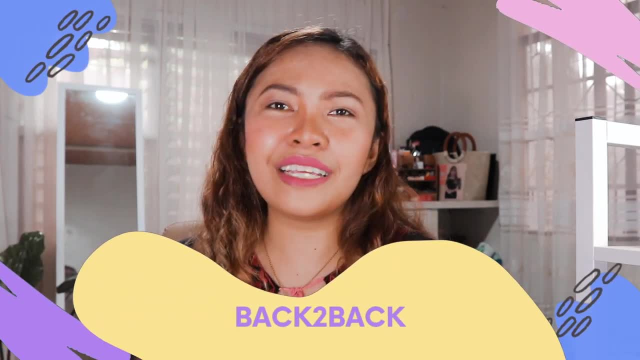 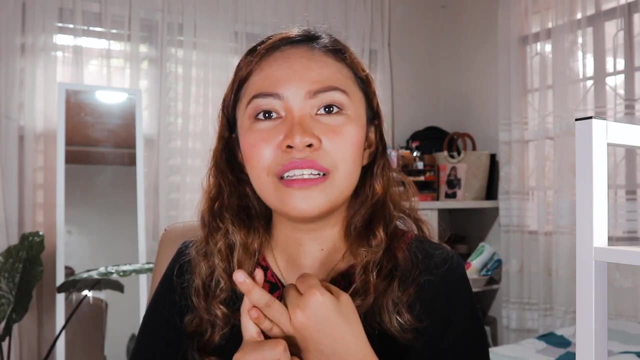 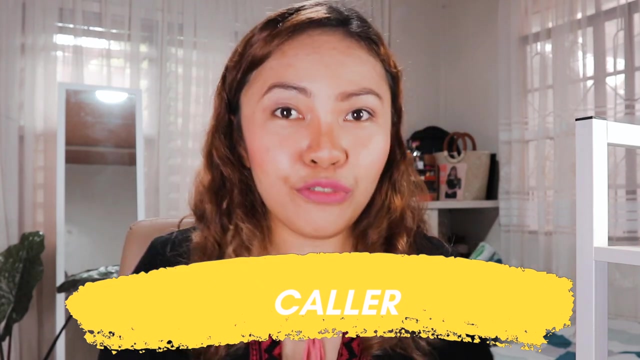 Number three is back to back. Supplies needed here are just minimal. All you have to provide would be a writing surface, writing utensils and someone who is quick with their math facts as a caller. So if you're part of that back-to-back tandem, the goal of this game is for you to guess. 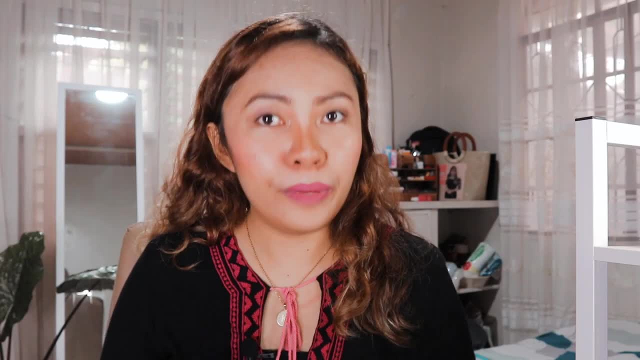 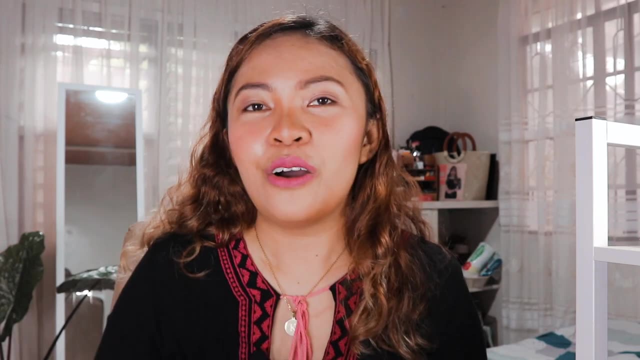 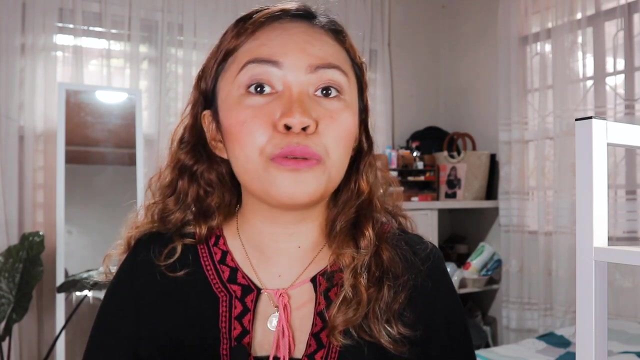 the other player's number before they guess yours To play. two students come up to the board and answer back to back. That's why the name is back to back. Okay, this position allows the students to write on the board, but blocks their view of the other person's number. Then here comes the. 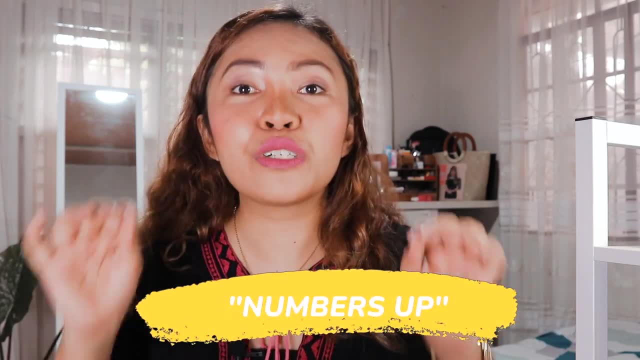 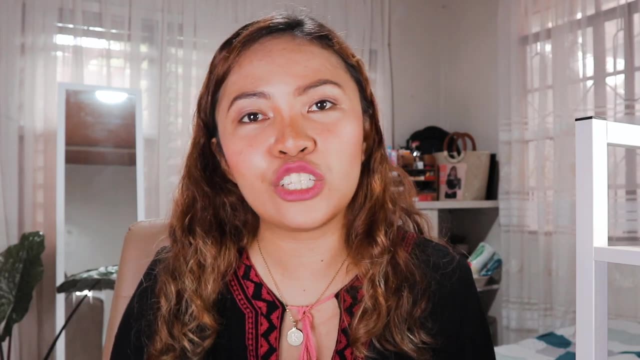 caller. The caller will state numbers up. This signals the two students to write their number on the board. I personally suggest that you ask students to choose numbers between two to nine to keep them from dwelling in the back of the board If you're part of that back-to-back tandem. 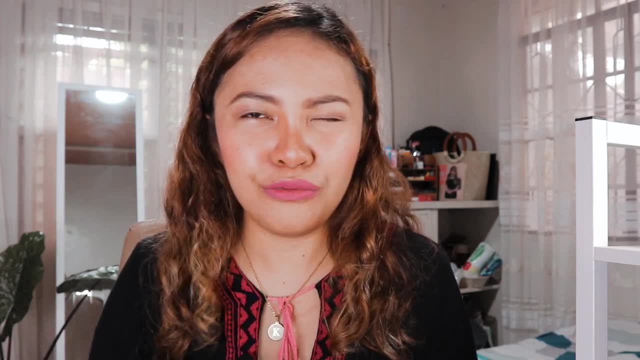 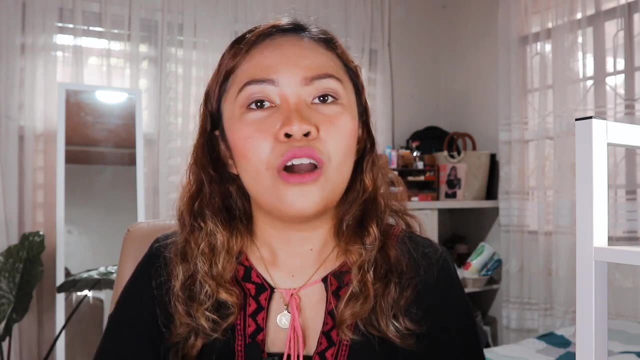 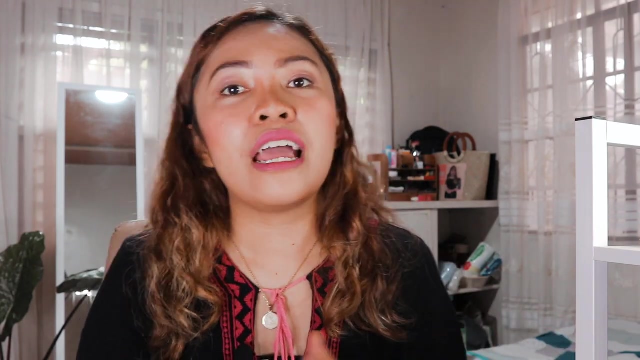 you can use the zeros and ones, which makes the game very, very easy, But you can always play with numbers, high or low, depending on the level of your students. Okay, so once the two are done, writing. the caller then states the sum for younger students or the product for older students. Again, 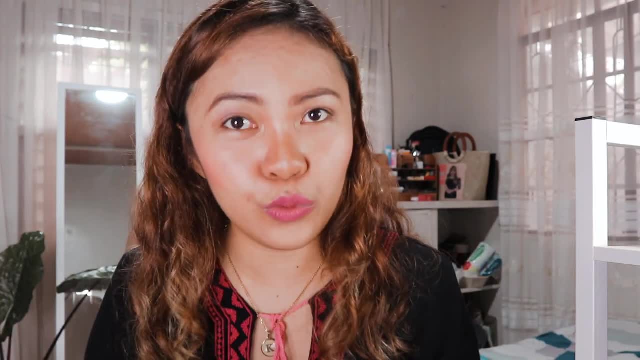 it's either the sum of the two numbers or the product of the two numbers. The students will then use their understanding of the math facts to figure out how to guess the number of those two. The students will then use their understanding of the math facts to figure out how to play. 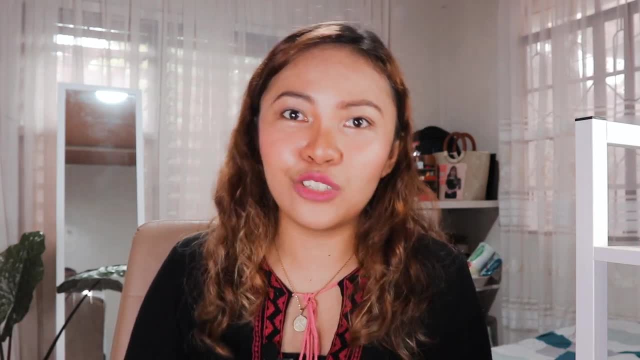 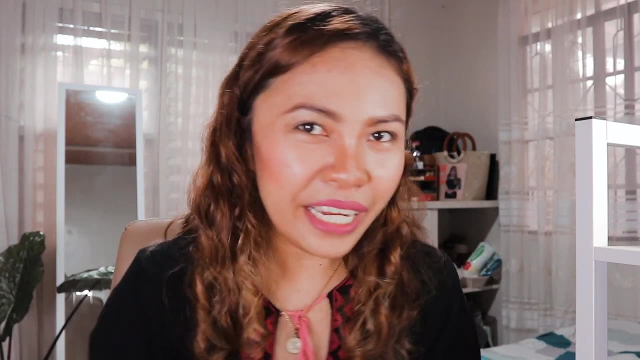 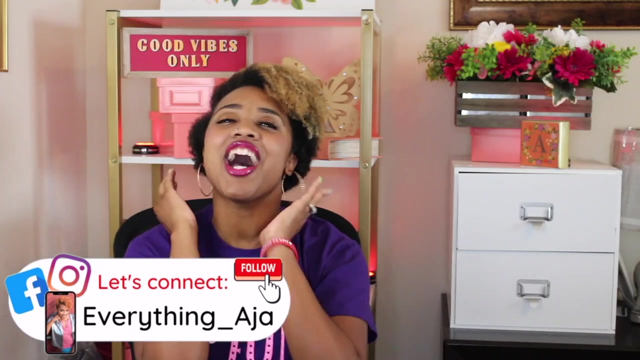 figure out what the other person's number is when added or multiplied. The first player to say the other person's number wins the round. Done with game number three. now let's call on Everything Adra for game numbers four and five. Math games are some of my favorite things to do. Not only do 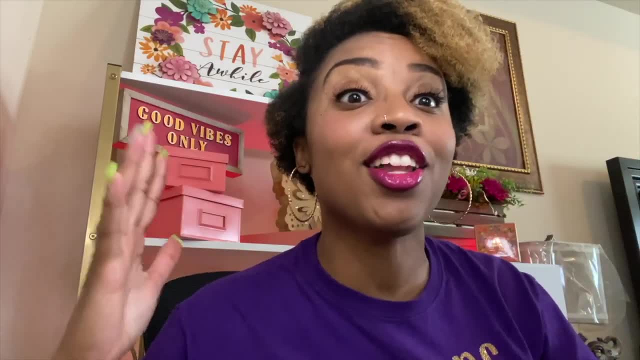 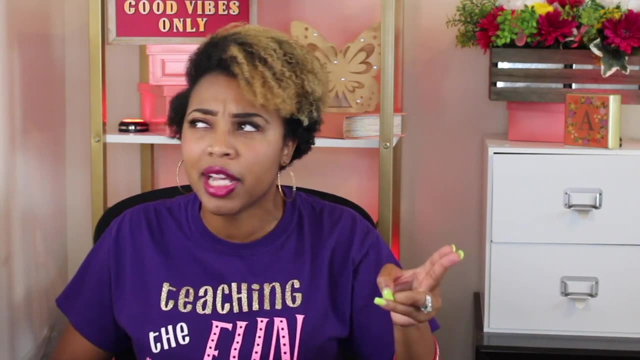 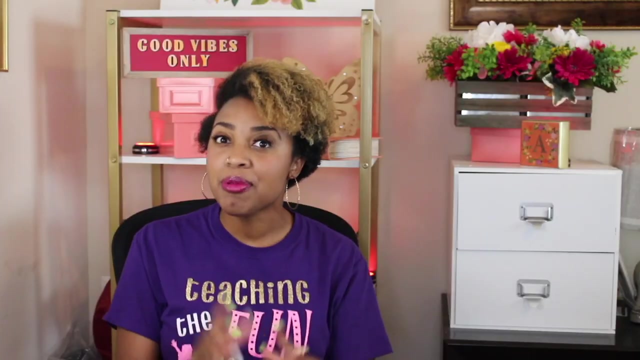 they help kids remember different math facts, but they also make learning fun. So let's talk about this Beat the Buzzer game. Beat the Buzzer is a digital game that can be played in person or through distance learning. In Beat the Buzzer, there are 10 rounds plus a bonus round. The object: 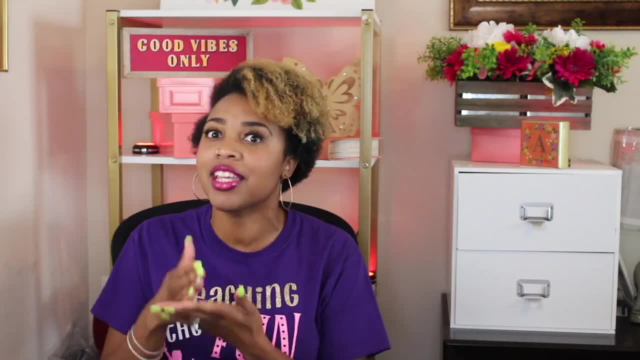 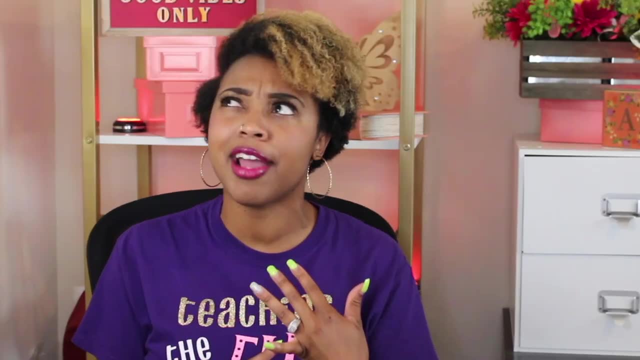 of the game for children is to actually make it all the way to the end of the game, thus beating the buzzer. Each round gets more and more challenging as the questions get harder and the time gets shorter. Now there is a little cushion in the game, because kids are able to miss up to two questions. 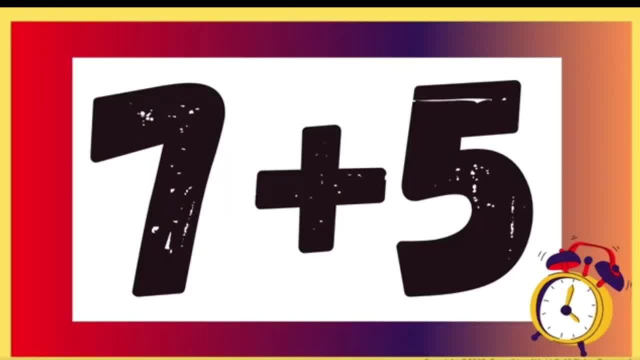 per round. You can also make this more challenging, and let them only miss one question. That is totally up to you. Now I actually have six different versions of Beat the Buzzer. I'm going to show you how to beat the buzzer. First, I'm going to 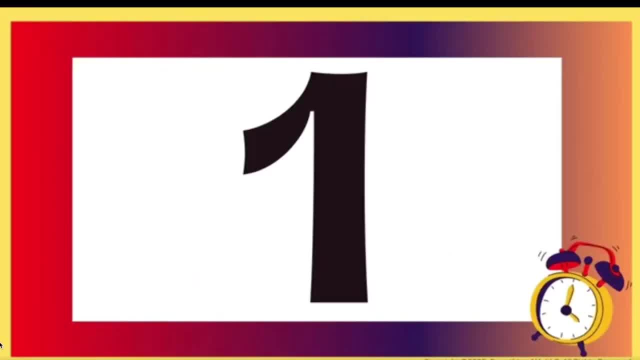 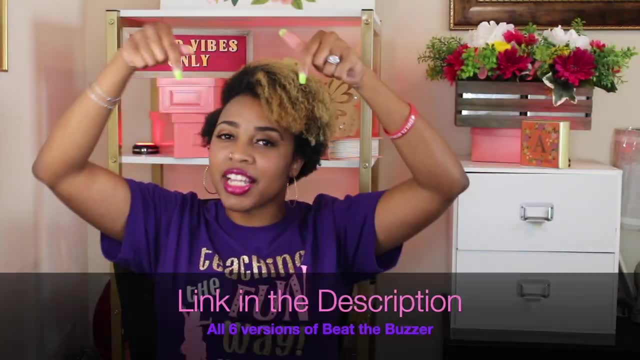 show you how to play the Beat the Buzzer game. I have number recognition, addition, subtraction. addition and subtraction, multiplication and division. If you want to find out more about the Beat the Buzzer game, then check out the link below in the description. Now the next thing. I